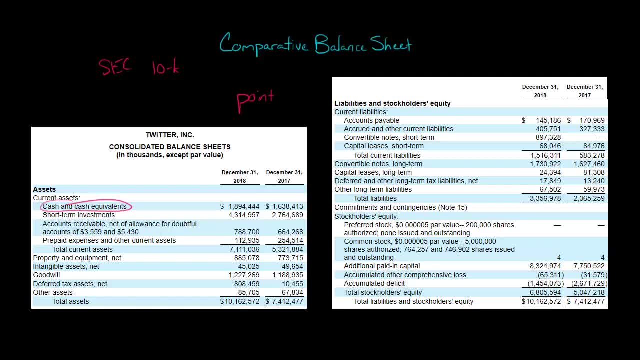 So this is telling us, for example, when we have cash and cash equivalents, it's telling us this is the amount that Twitter would have: just shy of $1.9 billion, because these amounts are in thousands- just shy of $1.9 billion of cash and cash equivalents as of 12-31-18.. 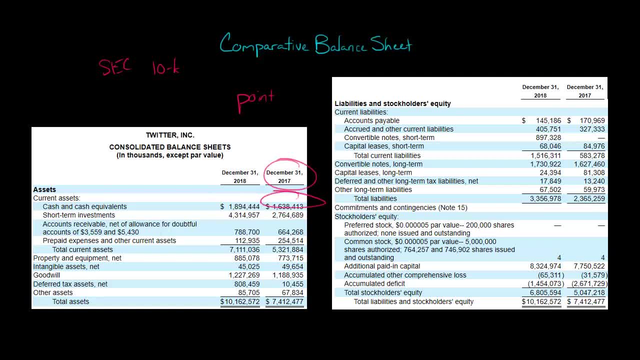 As of 12-31-17,, it was about $1.6 billion in cash and cash equivalents. Now, if you want to know why did the account change from one period to the next, you would go to this Statement of Cash Flows. 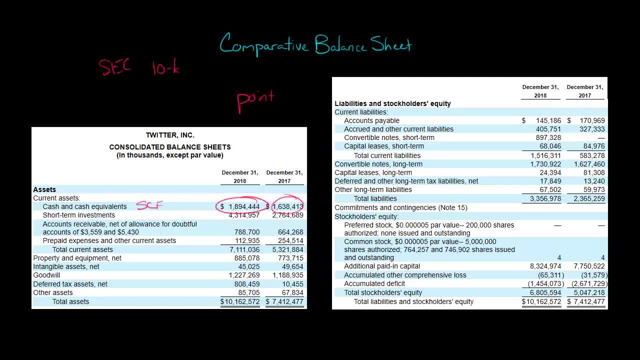 All we can see here with the balance sheet is cash went up, but we don't know why. Why did cash go up? Did they generate cash flow from their operating activities, from investing and so forth? So we go to the Statement of Cash Flow and that'll give us richer information. 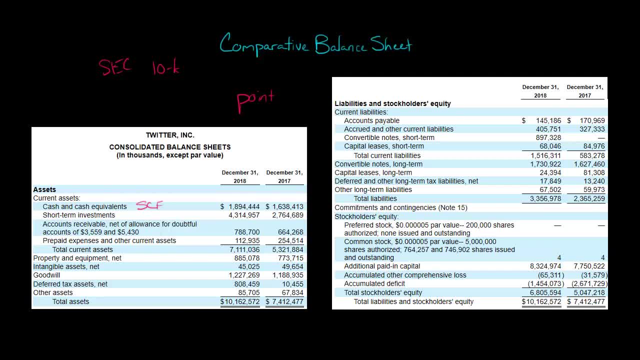 about why the cash balance changed. Now notice a couple things. with our comparative balance sheet, We're going to have where, in each case, total assets is going to equal total liabilities and equity. So here's for 2018.. Assets equal liabilities plus equity. 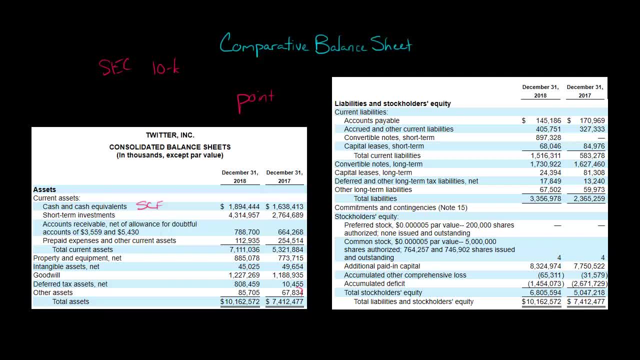 And then for 2017, it will be the same thing. We have a little over $7 billion in assets, $7 billion in liabilities and equity, So assets are always going to equal liabilities plus equity. Hopefully you know that by now. 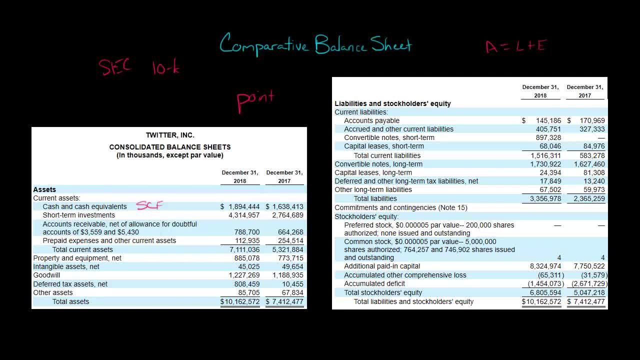 Now we're going to break out just like a regular balance sheet. we're still going to have it broken out into. we've got our current assets and then here. so here's our total current assets. Those are ones that'll turn into cash or be used within one year of the operating case. 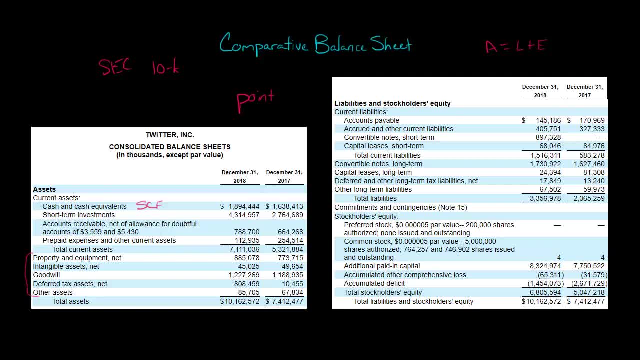 And then here all these accounts, these asset accounts are non-current. So this is our non-current assets. Okay, things like property, plant and equipment and so forth. And if you're wondering, well, what is in this property, plant and equipment? 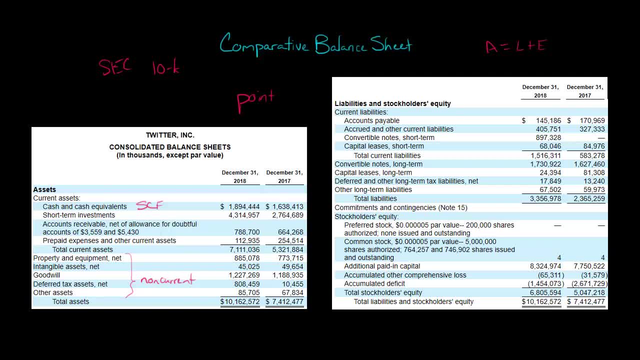 and how much accumulated depreciation was taken out and so forth. you would go to the notes, You would look up the notes and there would be a note on property, plant and equipment and tell you: okay, some of that property, plant and equipment is furniture. 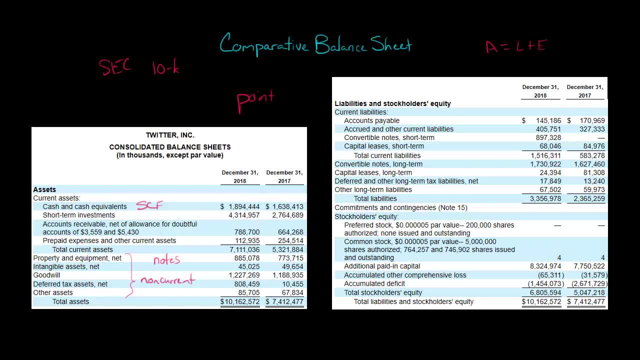 Some of the property, plant and equipment is something else, and so forth. Okay, so there's a note for many of these things. in the, for example, cash and cash equivalents, There is a note telling you what are some of the cash equivalents. 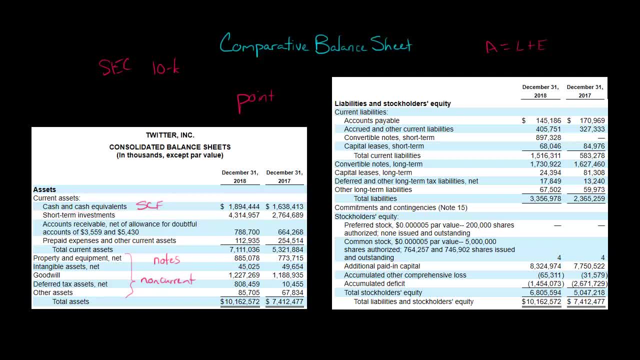 Do they have a money market account or so forth? Is it commercial paper? Okay, so we've got our current assets, We've got our non-current assets, and that equals up to our total assets. And again, we have it for one period or, excuse me, one point in time. 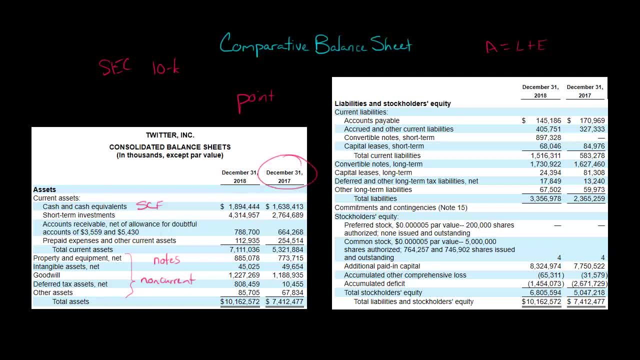 December 31st 2018.. Okay, and then for a second point in time, December 31st 2018.. So we basically have two balance sheets here instead of just one. Now, when we look at liabilities, you're going to see that there's current liabilities. 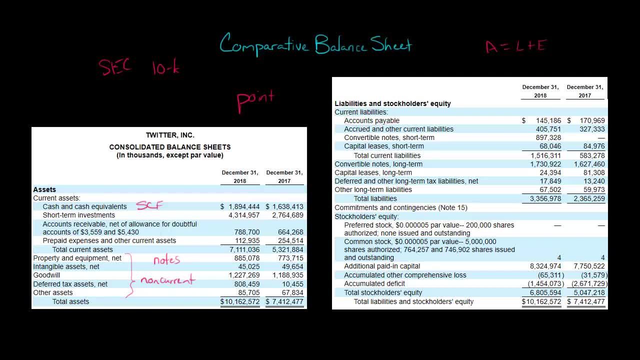 and we've got the usual suspects, things like accounts payable. Okay, we've got our current liabilities, but then we also, after total current liabilities are summed up, we have these accounts right here and these are going to be long-term or non-current liabilities. 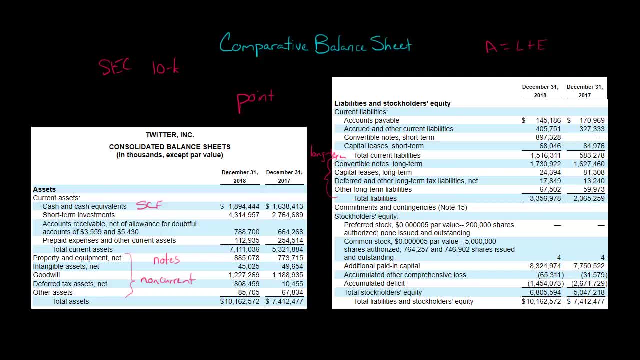 Okay, these accounts right here. Those are long-term liabilities. Now in our stockholders' equity section we're going to have preferred stock, common stock and so forth. That's money that the investors put up. Okay, we've got additional paid-in capital, all these things here. 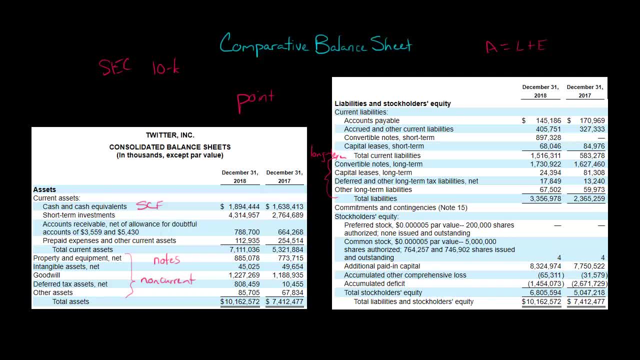 basically money that investors have put up invested in Twitter. Now we've got our accumulated deficit. We do not see retained earnings because retained earnings is negative. It has a debit balance. That means that at this point in time, as of December 31st 2018,. 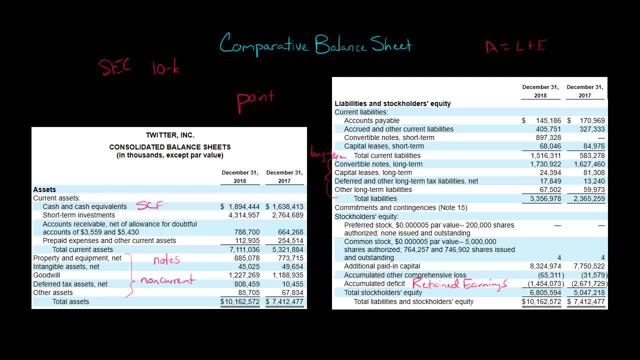 Twitter had accumulated more losses in the past than it had profits. Now we see our total stockholders' equity and then we've got our liabilities and equity. Now, if you want to know, for example- so let's say you're looking at the accumulated deficit- 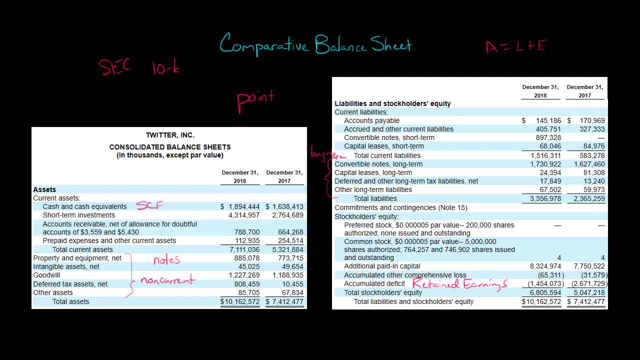 which again is what we call retained earnings, when retained earnings is negative and has a debit balance. If you want to know why, did it change from 12-31-2017 to 12-31-2018, which we see that it went down significantly? 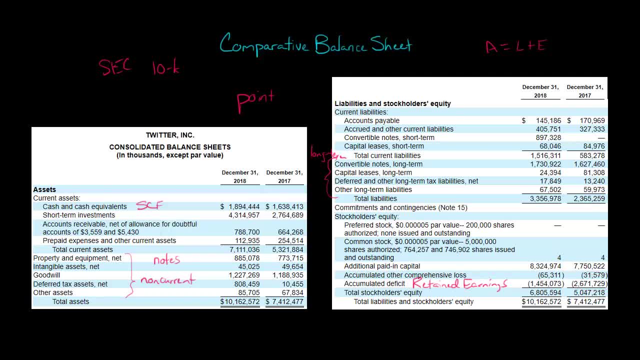 the accumulated deficit over $2.6 billion. we'd go from $2.6 billion of accumulated deficit to just $1.4 billion. If you want to know why it went down, you would go to the statement of stockholders' equity. 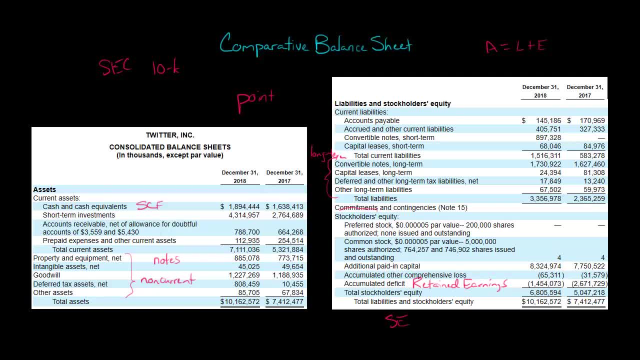 Remember, that's one of our major financial statements. You go to the statement of stockholders' equity. In fact, the statement of stockholders' equity would tell you why all of the equity accounts change If, for example, additional paid-in capital changed. 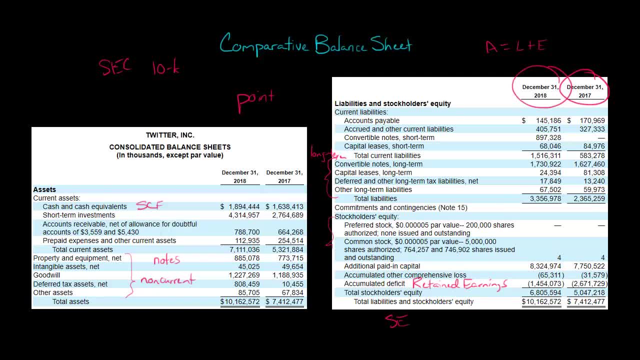 from this balance sheet date to this balance sheet date. so you would go to the statement of stockholders' equity and you could see: Okay, why did it go from $7.7 billion to $8.3 billion, and so forth. 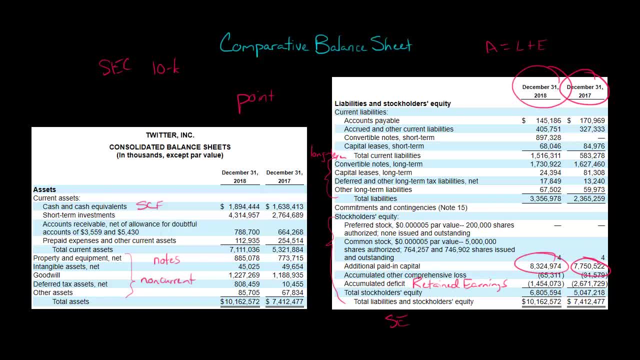 And it'll delineate in more detail why the company's amounts changed from one balance sheet date to the next. 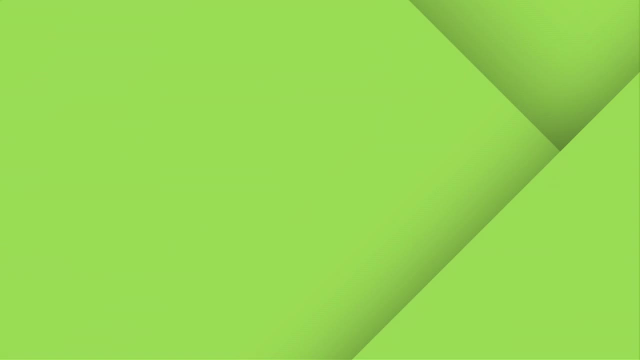 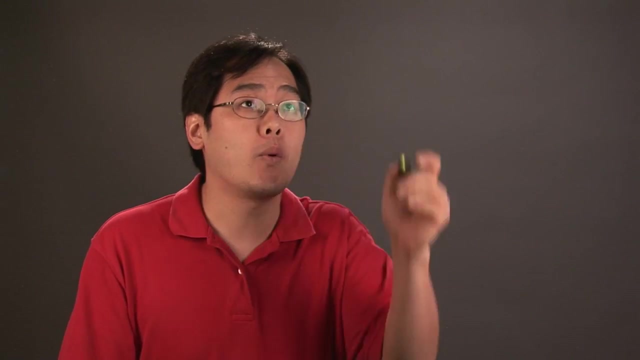 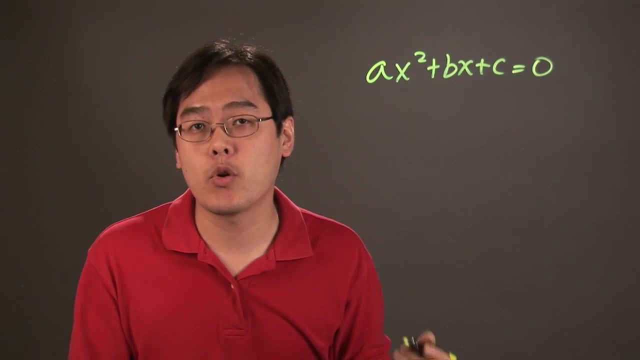 Hi, I'm Jimmy Chang, and we're here to talk about how to solve quadratic equations. for a radical, Now, as you know, with a quadratic equation it's of the form: ax squared plus bx plus c equals to zero. That's the form of a quadratic equation. Now, the thing is, though, if you have, 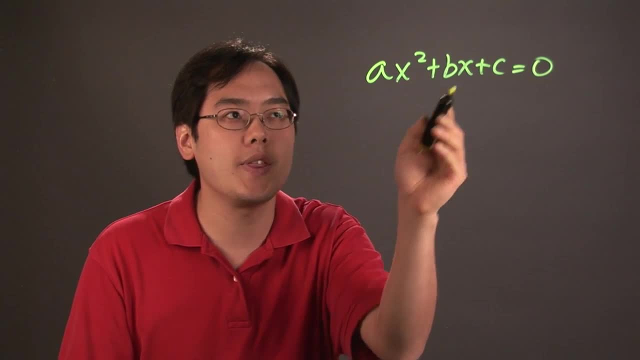 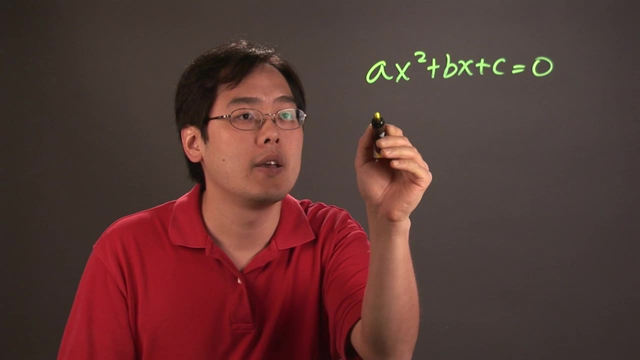 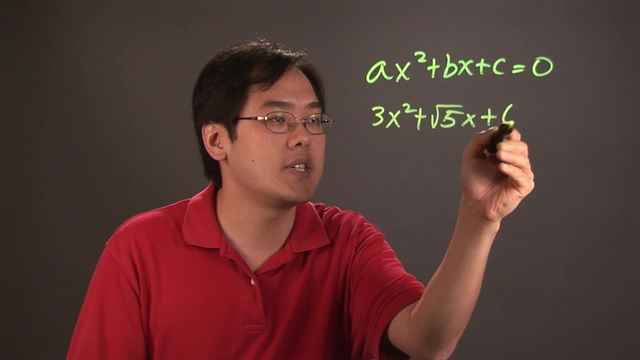 radicals involved. the radicals probably shouldn't really appear where the x's are. So where you might get it is in the coefficients. So, for example, if you have something like, let's just say, 3x squared plus square root of 5x plus 6 equals to zero, what you might contend. 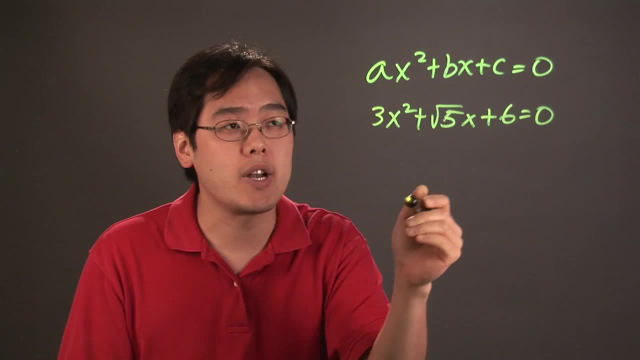 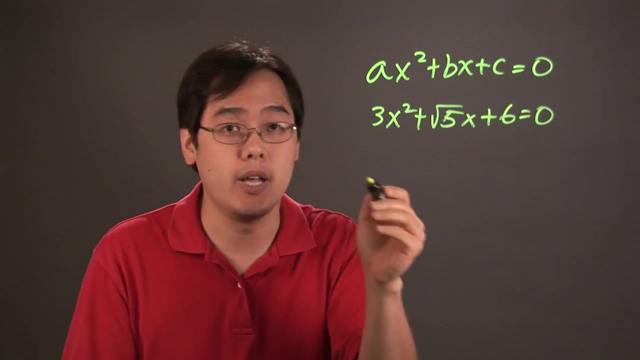 with sometimes is being able to use the quadratic formula to solve it because, as you can tell, it's not really factorable, but being able to use these radicals in the quadratic formula. Now, as a friendly reminder, you know it's negative b plus or minus square root of. 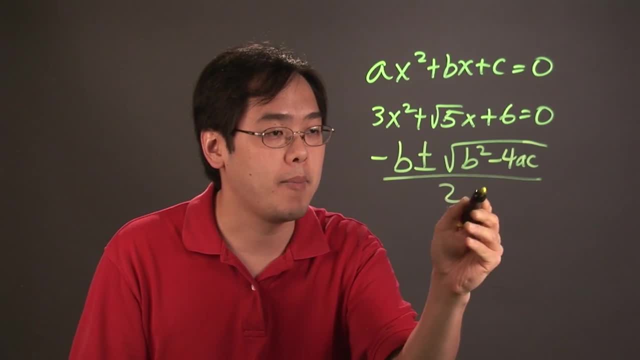 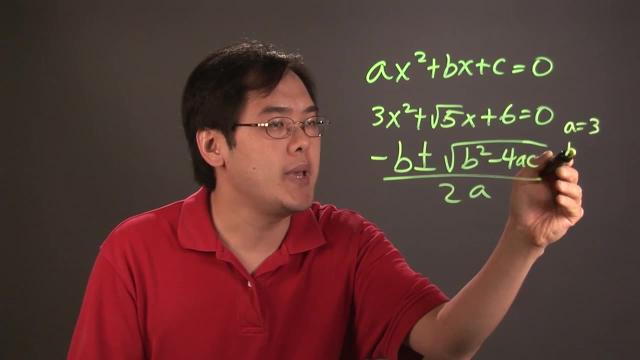 b squared, So you might get it is where in the coefficients. So, for example, if you have b squared minus 4ac over 2a, Now where you incorporate these radicals is just plug them in where they belong. So you know, a is 3, b is square root of 5, and c is equal to 6.. 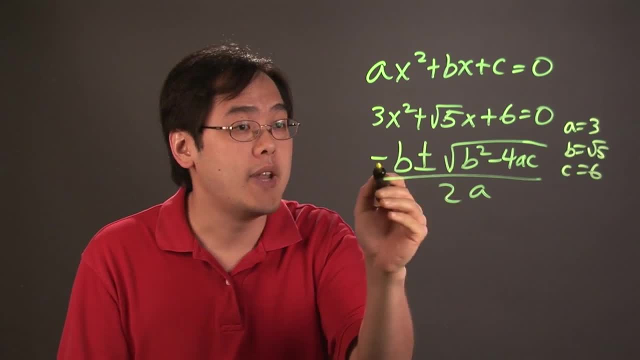 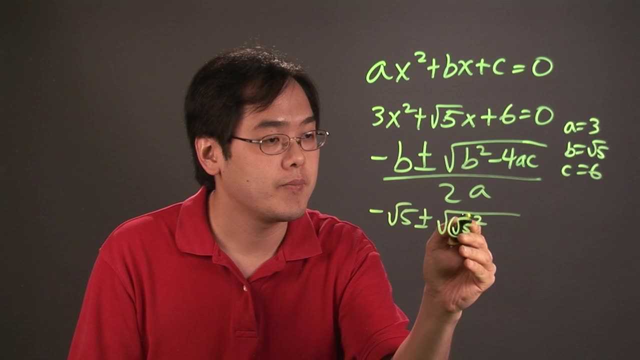 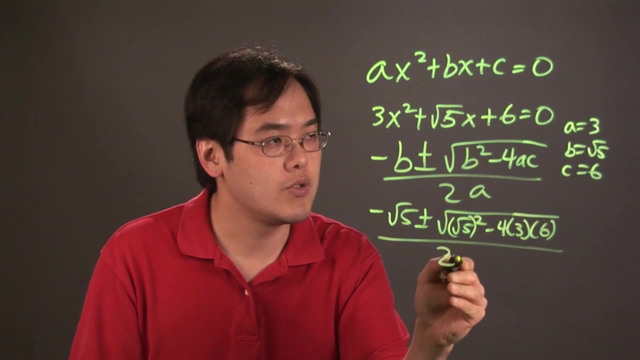 And all you need to do is plug them in. So negative b is negative. square root of 5 plus or minus. square root of square root of 5 squared minus 4 times a is 3,, c is 6.. Over 2 times 3.. And what all it is now is just strictly algebra: You have negative square root. 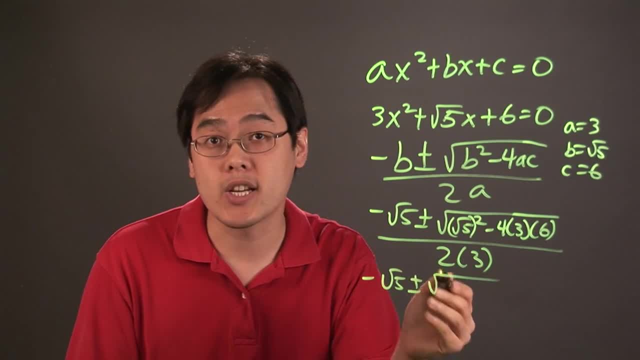 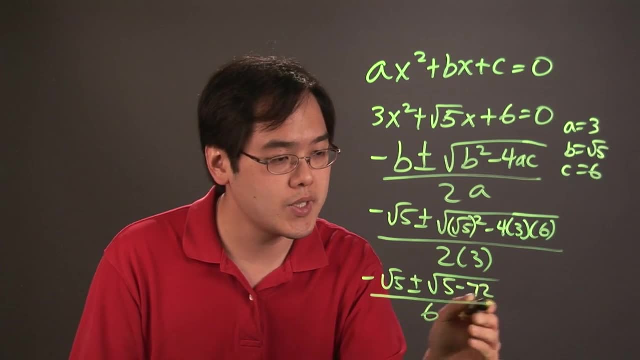 of 5 plus or minus. Now, square root of 5 squared is actually 5 minus 4 times 3 is 12.. 12 times 6 is 72 over 6.. And so you have negative square root of 5 plus or minus square root of negative.